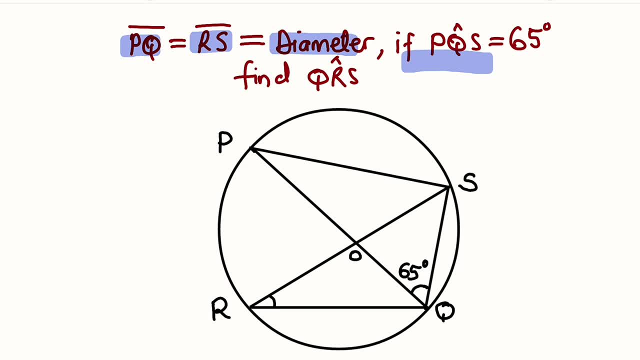 It says that if angle PQS is equal to 65 degrees, find angle QRS. This is angle QRS. Let me mark it as X. Alright, once you master the laws on the cycle theorem, you will find it very simple to answer this question within a minute or less than that. Okay, let's get started. 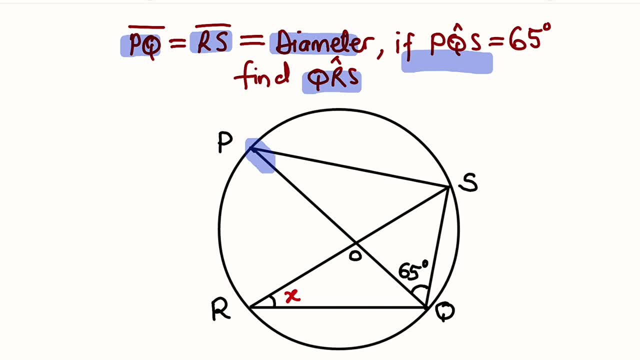 From the question it mentions that this line right here is a diameter and from one of the laws it says that if a diameter form an angle to the circumference, that angle form is 90 degrees, So you can see that we have an angle here formed by that diameter. So we can make it clear that this angle right here 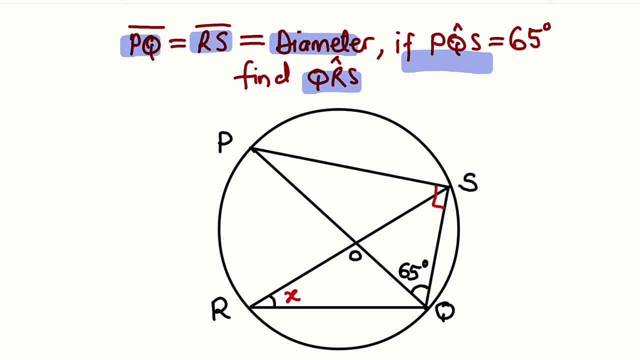 is 90 degrees And if it is 90 degrees, the whole of this triangle. PQS is said to be a right angle triangle And if it is a right angle triangle, by adding this angle right here to this angle right here, we are going to obtain 90 degrees. Therefore, this angle will be 25.. 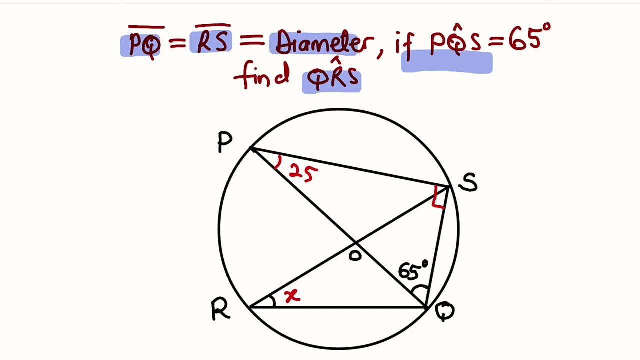 degrees, because if you add 25 to 65, you are getting 90 degrees. We are almost done. Consider this line SQ. It is a code And that is a law that says that all angles formed from the same code to the circumference are equal. Can you see these two angles? Angle R is formed. 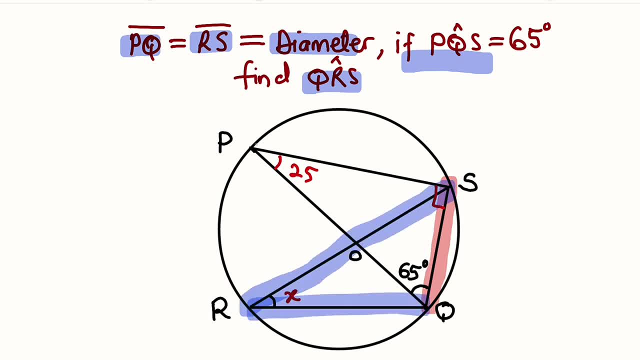 from that code. Likewise, angle P is also formed from the same code. Therefore, angle P and angle R are said to be equal. Therefore, X will be equal to 25 degrees, And remember this. X is our angle. QRS, which we are looking for, equals 25 degrees, And this is our solution. 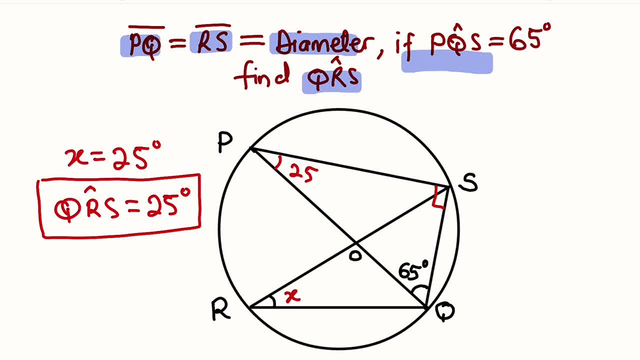 The angle we are looking for is 25 degrees, And this is all I have for you today. Thank you for watching. Do share to your learning colleagues and don't forget to subscribe to my YouTube channel for more exciting videos. Bye, bye.